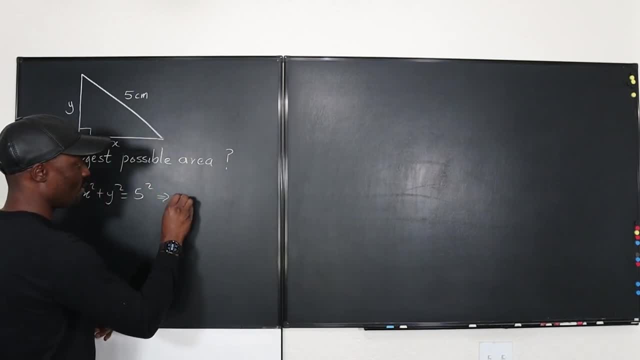 only So what do you think y will be? This implies that y squared will be equal to 25 minus x squared, which means y equals the square root of 25 minus x squared. Okay, 25 minus x squared. So here let's write the formula for the area. Remember, area is half base times height. 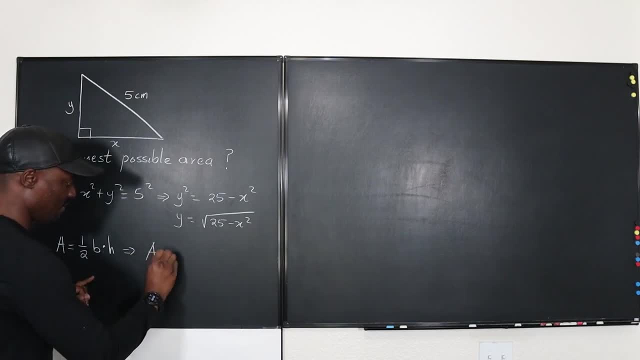 okay, and this implies that the area we're looking for will be one half of the base. The base is x and the height is going to be y. okay, But this y is what I'm going to put here. but I'm going to 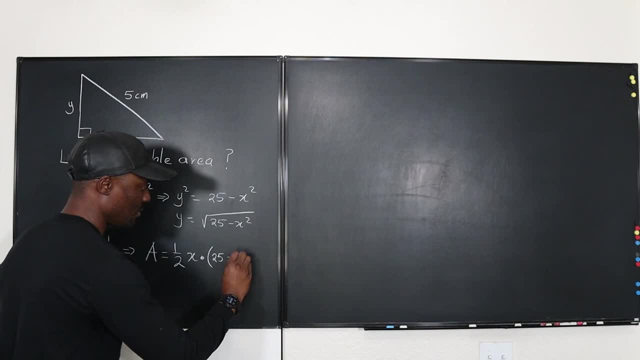 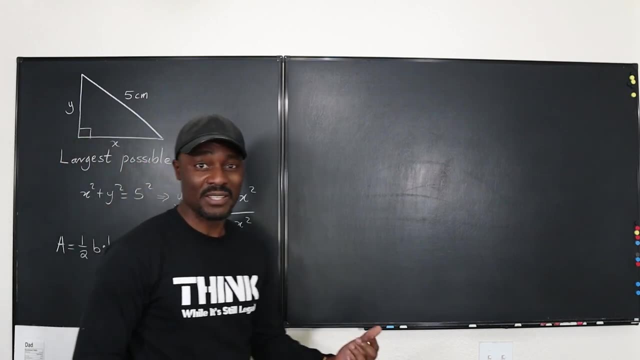 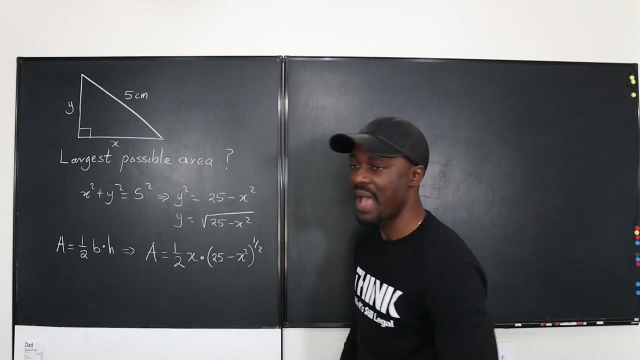 write it this way. I'm going to write it as 25 minus x, squared, raised to power one half. I wrote it this way in the exponent form so it's easy to differentiate. So now we want to find the maximum area. What will x be for this to be maximum? So our intention is to maximize, So our plan. 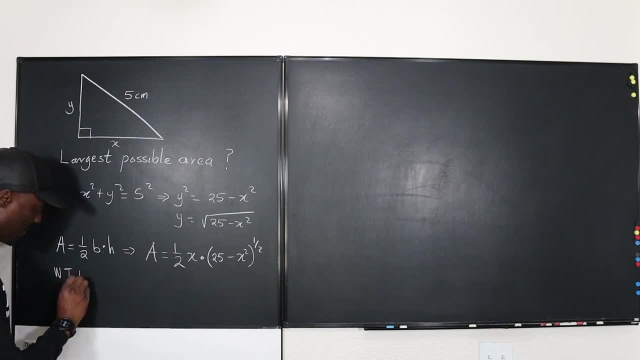 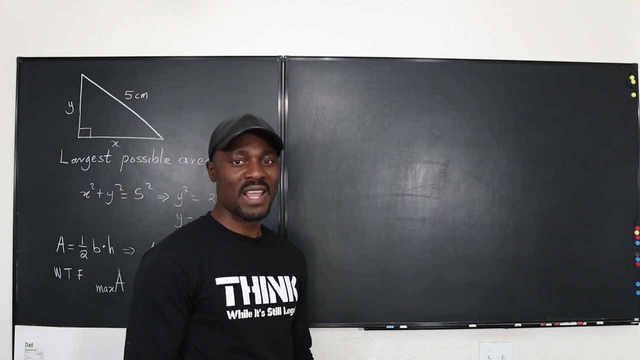 we want to find maximum a. okay, We want to find maximum a, which will be: and that's what happens when you take the derivative, you equate it to zero, find the critical number and that's it, Okay. so let's do that. What will d a, d x be? 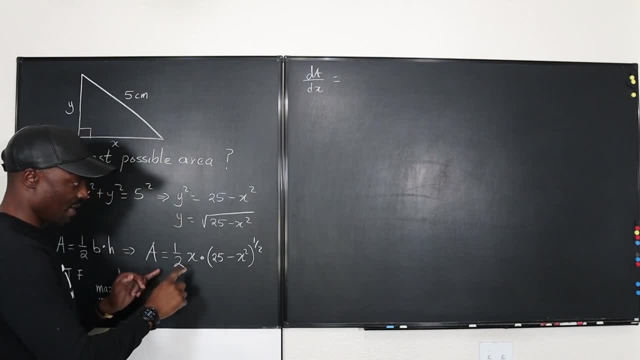 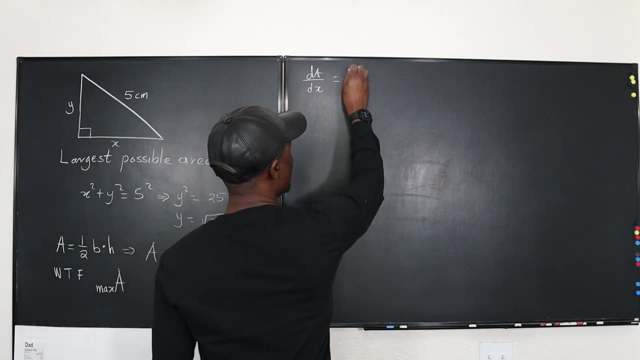 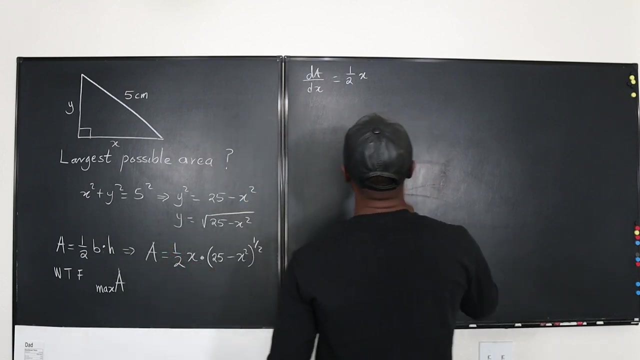 Okay, if we differentiate a with respect to x, we'll have to apply the product rule, because this is a product of two functions of x. So we follow the rules for product rule. You keep the first one half of x. you keep the first. you differentiate the second If I 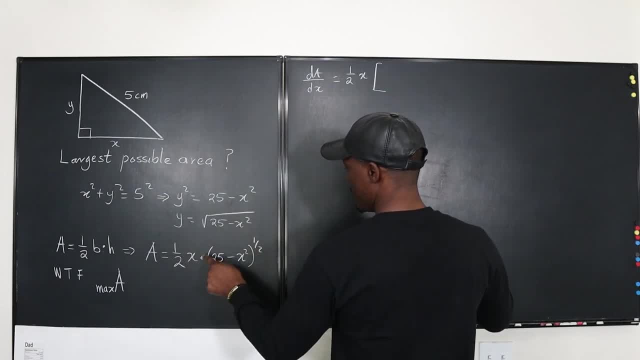 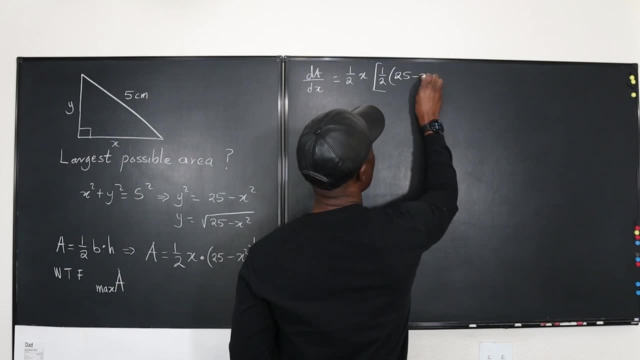 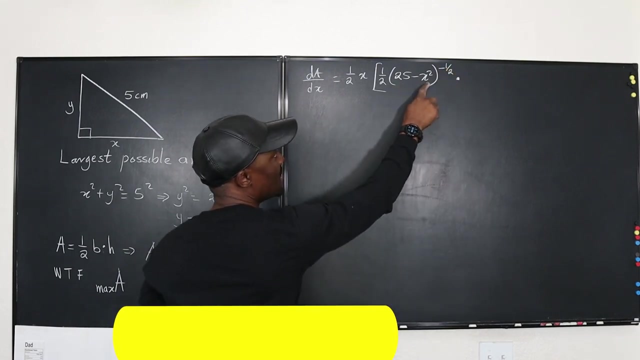 differentiate this. what I'm going to have will be bring down the one half. it's going to be one half, put in parenthesis, 25 minus x, squared raised to power. subtract one from this negative one half, multiplied by the derivative of the inside. 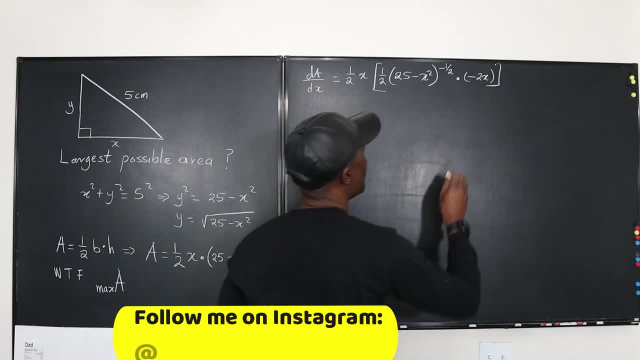 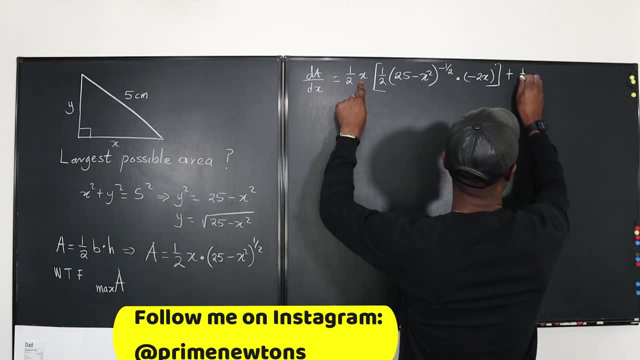 which is negative, two x. Okay. so all that is the first step of the product rule. The second part is add. we differentiate the first, that's going to be one half, and then we keep the second. The second is just this function, that's going to be 25 minus x squared, raised to one half. 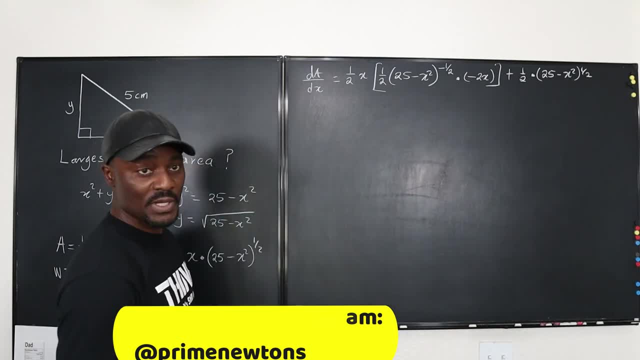 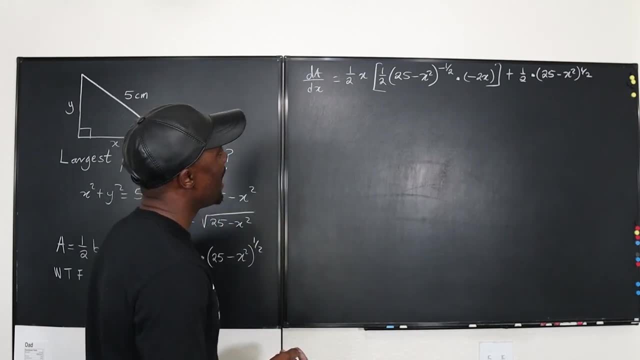 okay, so let's do the cleanup. this is where most people so the calculus is done. this is where most people get stuck. it's in the cleanup. I know that if I multiply this one half or this one half will take out this one, so there's gonna. 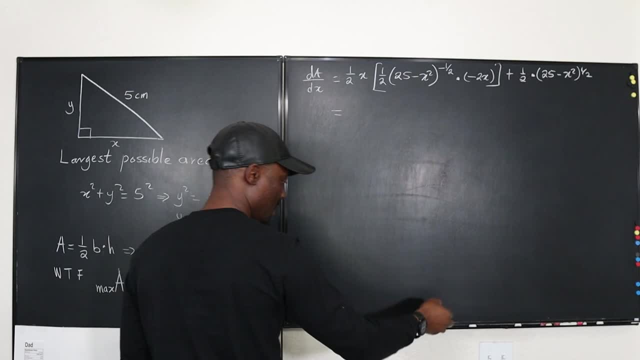 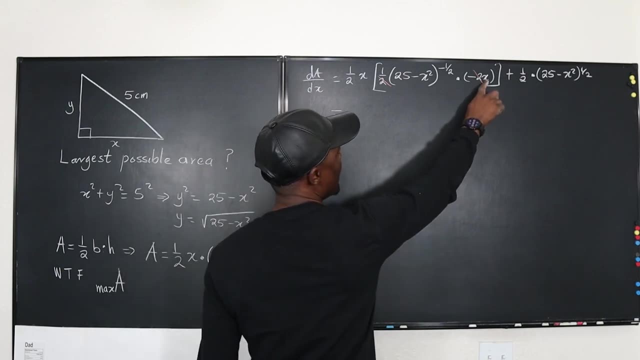 be a negative. eventually. that comes out okay. so let's start canceling. so I'm gonna cancel this two. with this two and what I have, I'm gonna have an X and then another X and this half remains. so I'm going to have one half of x squared. 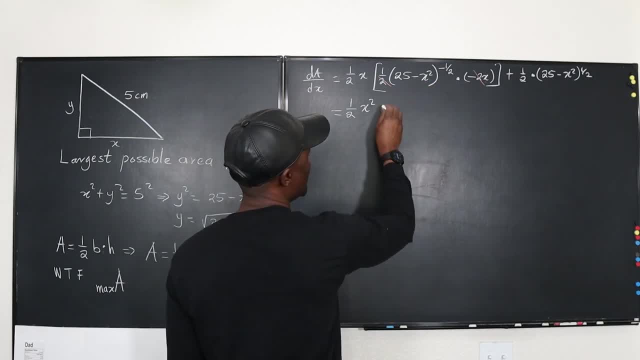 definitely, and then I'm going to have this expression: that's all that's left. so it's going to be 25 minus x, squared to the negative one half, okay, and if I go here, it's going to be plus. there's nothing, I'm just going to have one half. 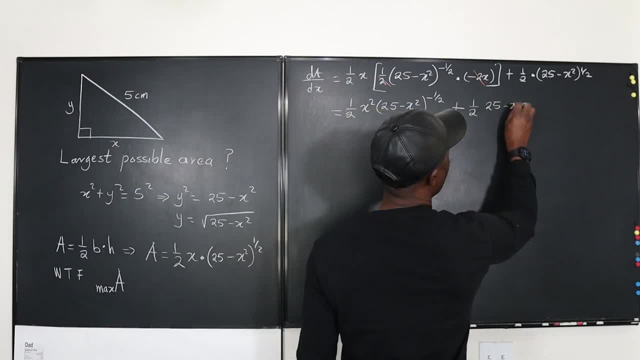 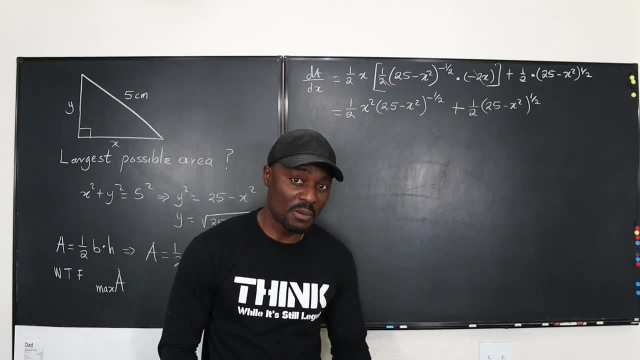 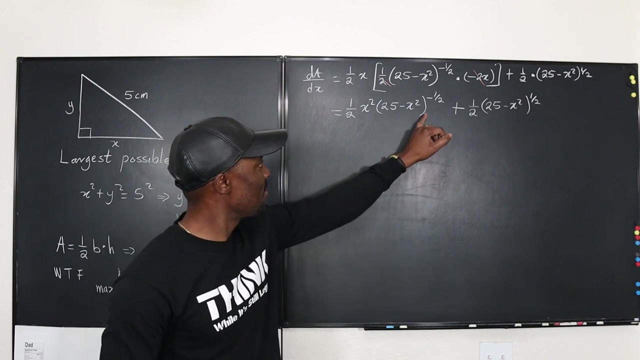 also of 25 minus x, squared to the one half. okay now, because I need to find the critical number or I need to solve for X. it is always easier for you to put the two together. write them, because this is gonna be a fraction, as you can see, so I can. 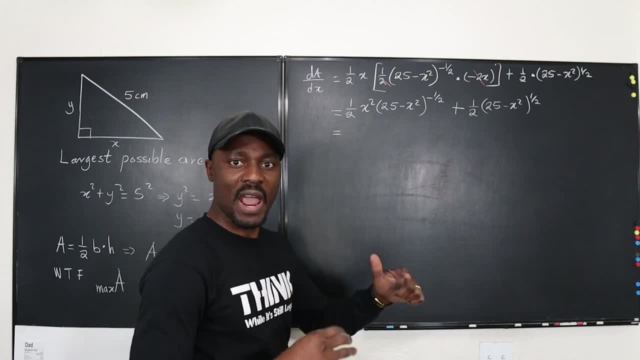 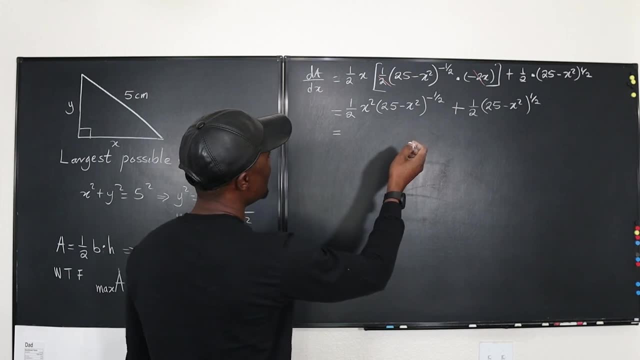 transform this back to a fraction. if you bring this down because it has a negative exponent, you're gonna have this become. there was a negative. where is it? oh, I converted it to equal sign. no, okay, there's a negative here that came out of that out. So we're going to have the negative of x squared here, okay, And under I'm going to have 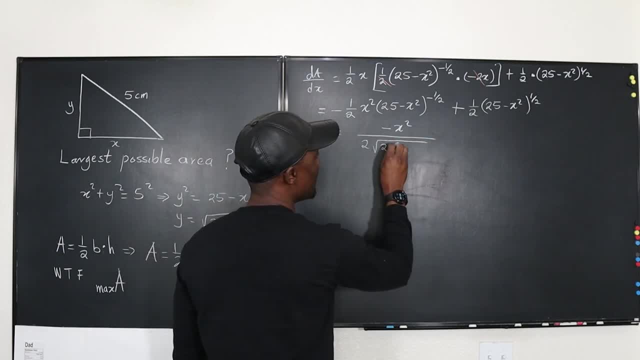 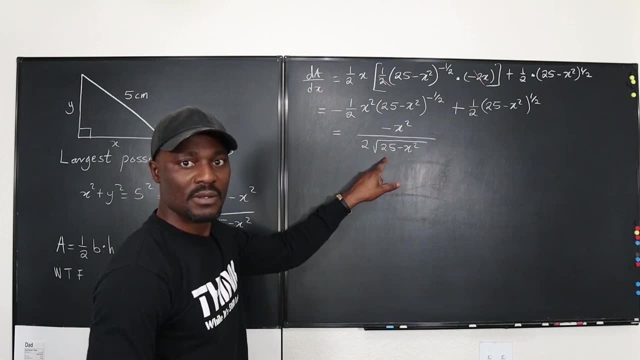 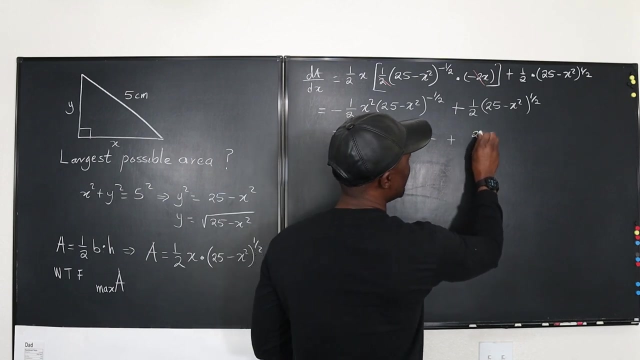 2 times the square root of 25 minus x squared. okay, Take a good look at this. This is what this means. okay, Plus, I'm going to have just this: It's going to be 25 minus x squared the square. 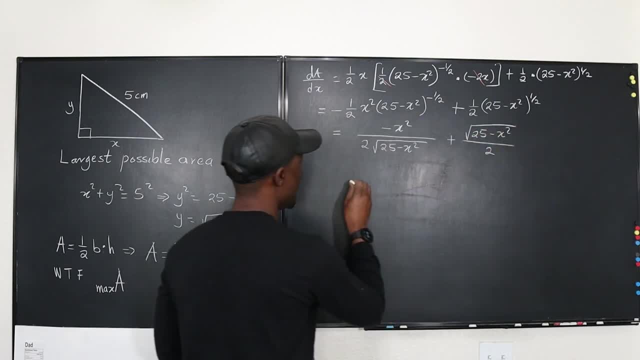 root divided by 2,. okay, Now, if we put these two expressions together, this has 2, this has 2, definitely I'm going to have a 2 under. and this has square root of 25 minus x squared 25. 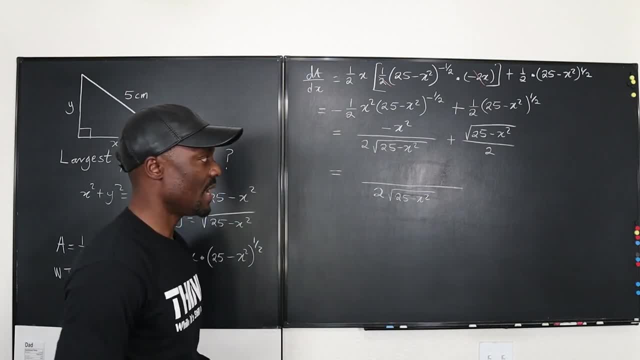 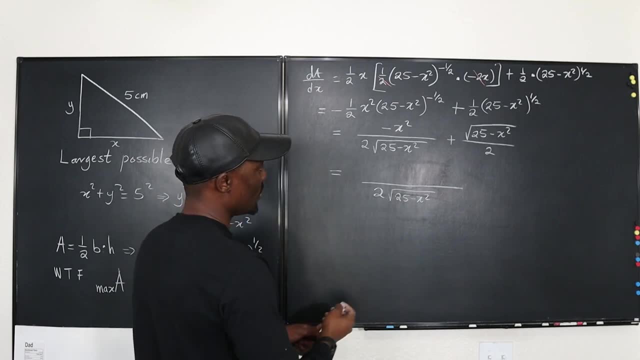 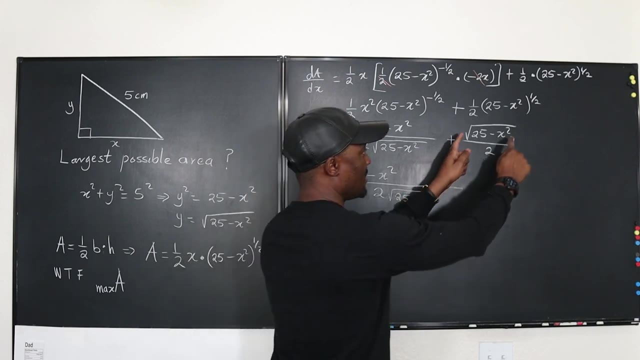 minus x squared. okay, And on top, what do I get? I get: so this and this, this is going to be exactly negative x squared, and this and this is going to be this. If you multiply this by this, you're going to get just this times, this is going to remove the square. 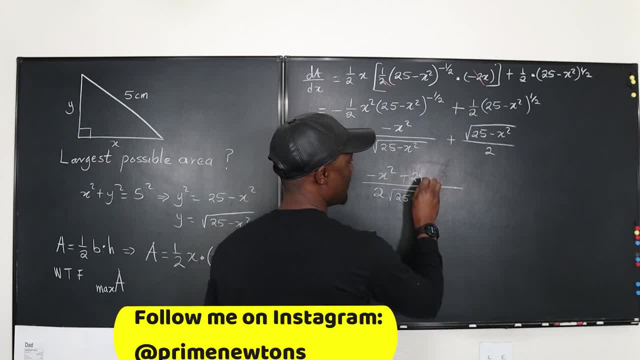 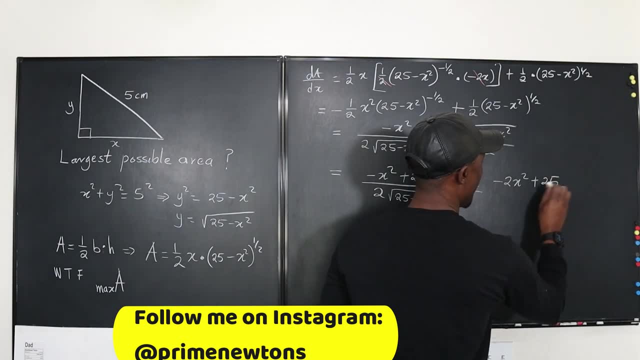 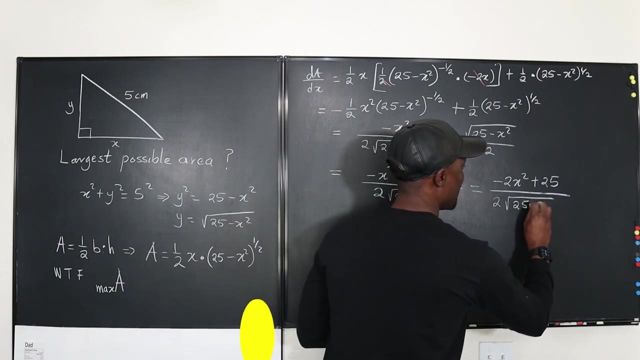 root and then you have just 25, so that's just 25 minus x squared. On top I have negative 2x squared and then I have plus 25.. And under I have 2 times the square root of 25 minus x squared. 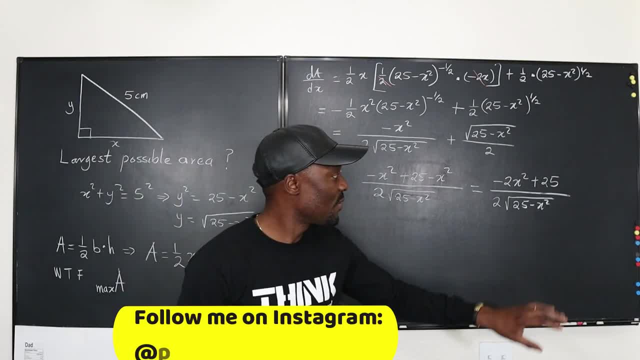 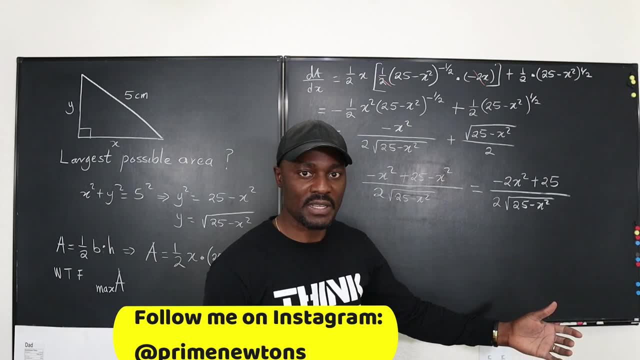 So now I need to find the critical numbers. Remember that for a rational expression, when you have critical numbers, they are the values of x that make the expression zero, okay or undefined. So if you look here, what will make this zero will be when you equate this to zero? 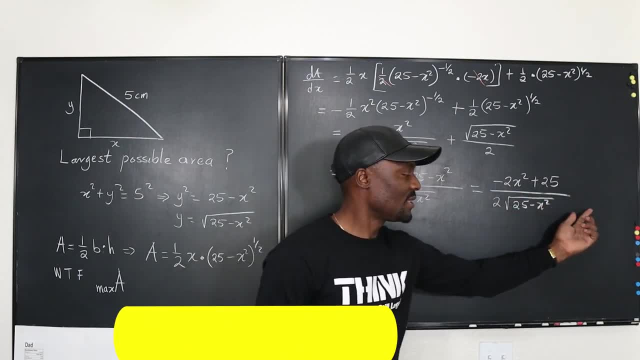 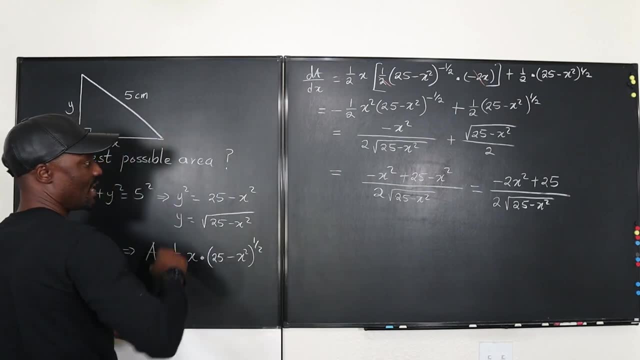 and when you equate this to zero? Well, when you equate this to zero, let's take both of them. So what we have is: so let's investigate critical numbers. I think I'll have to do this here, but I'll write the answer eventually here: Critical numbers. 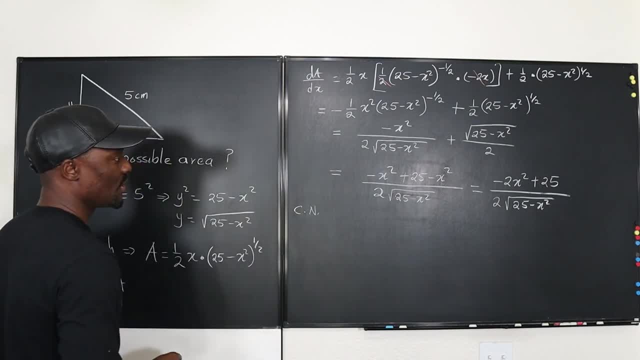 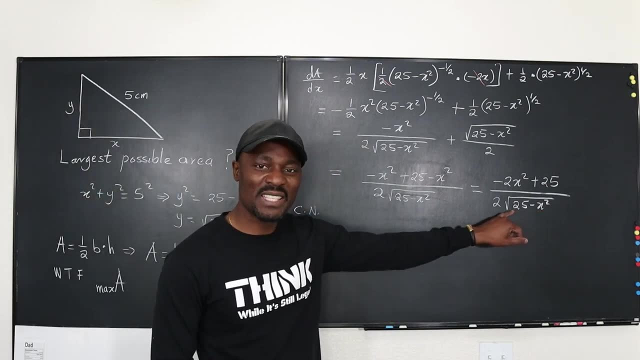 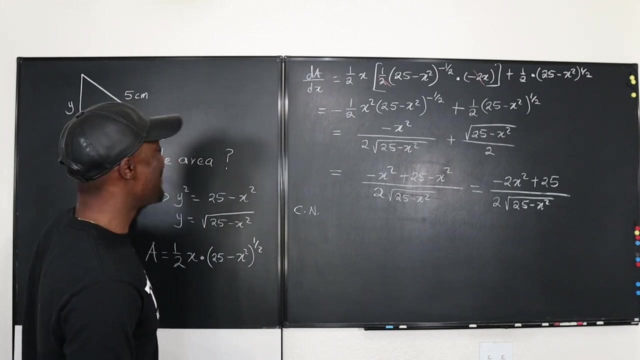 Okay, will be such that you have x being equal to. I can see that if I solve this, I'm going to get x equals 5,, which doesn't make any sense because x cannot be 5,. okay, If x is 5,, then it means y. 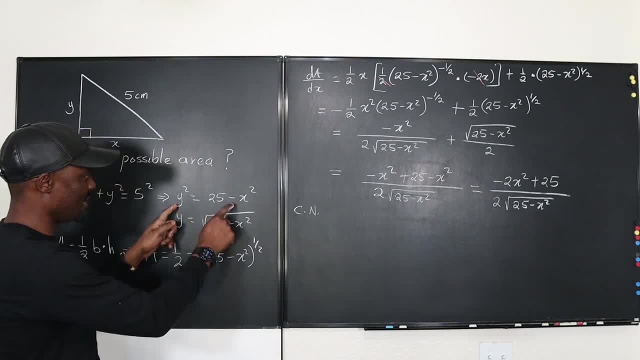 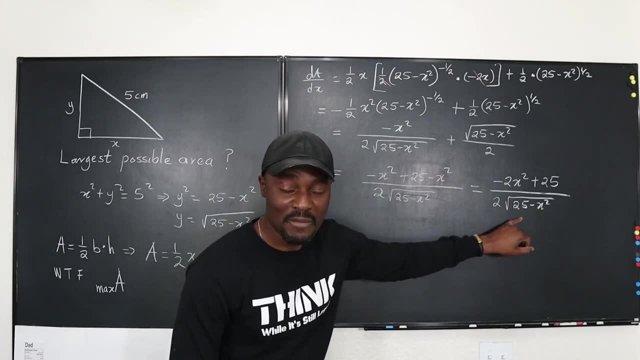 does not exist. As you can see, y will not exist and means there's no triangle. So I'm not going to be looking at the bottom, I can see it already, because solving this gives you x equals 5, and you can't use x equals 5, because it will make. if x is 5, then this is 5 squared plus y. 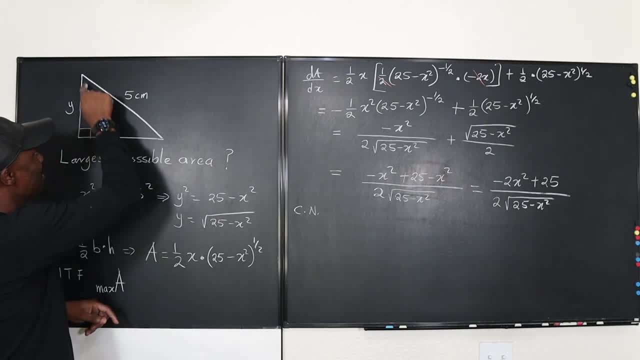 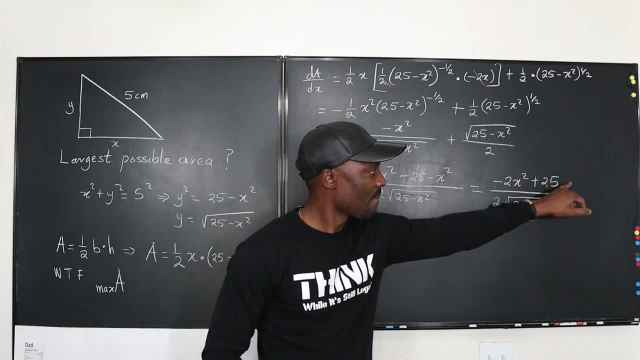 squared is 5. squared, It means y. squared is zero, which means there is no y, which means there is no triangle. So it's a no-no. But if you solve the top- look at the top- what you're going to get. 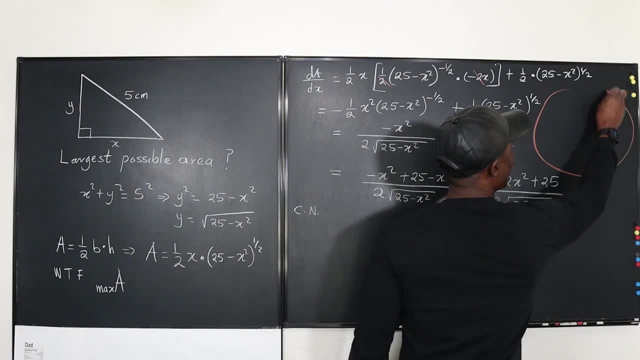 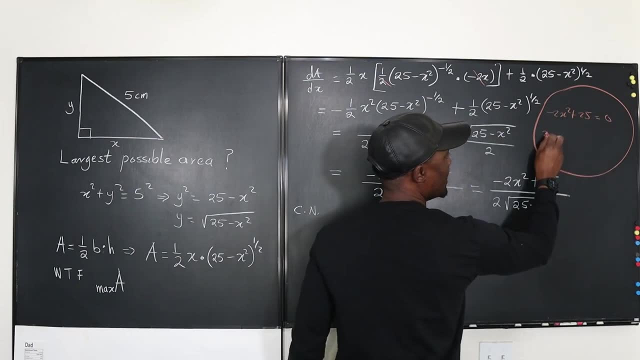 is. let me do it here. What you're going to get is negative. 2x squared plus 25 equals zero. That tells you that x squared has no triangle. So if you solve the top, look at the top- It has to be 25 over 2, which means x is the square root of 25 over 2.. I'm going to leave it. 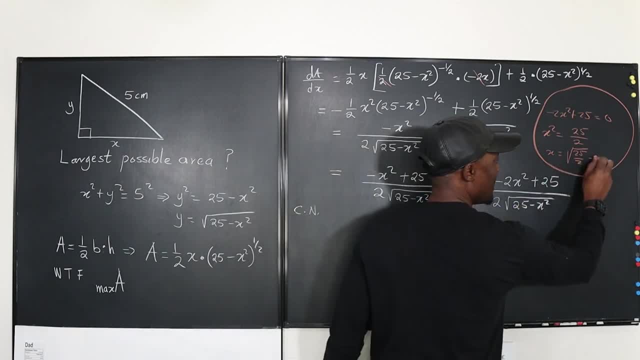 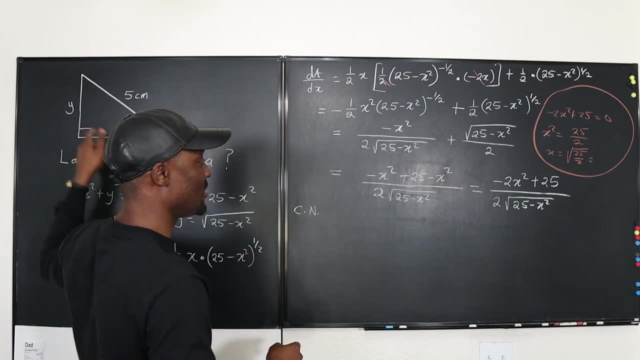 that way, not simplified, or I can simplify it. Well, this is going to be the same thing as see. it's supposed to be plus or minus, but I will not take the minus part because I'm dealing with the sides of a triangle and there's no negative portion. You see how you eliminate possible. 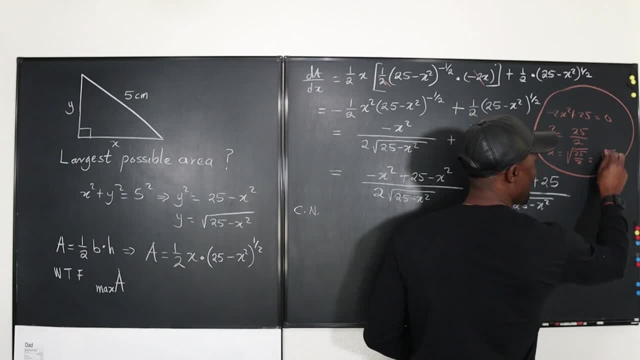 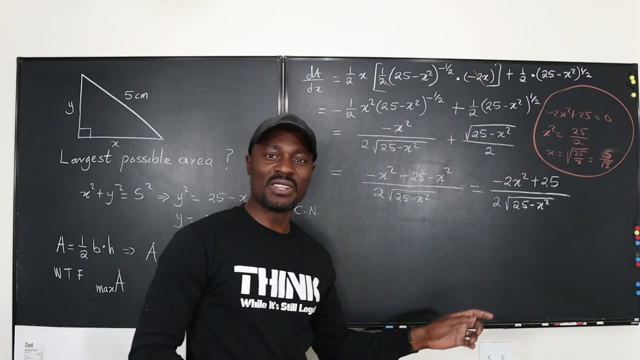 answers quickly, Okay, So what you do now is say this is the square root of 5 over- sorry, it's 5, divided by the square root of 2.. Now do you want to rationalize? Because really that's not the. 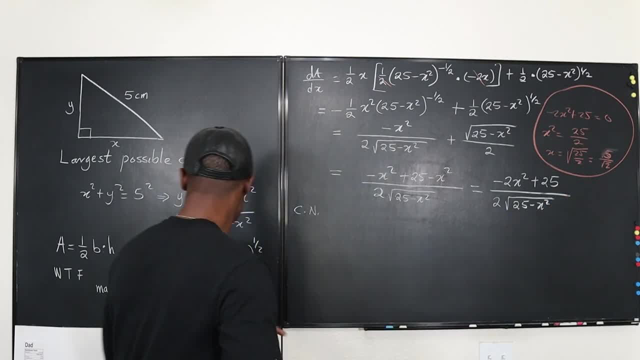 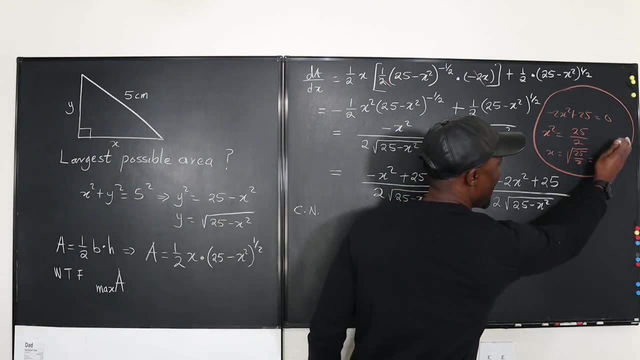 point of this exercise. You don't need to rationalize, because what we need is what would be the largest possible area. You're still going to use that number to calculate, So this is what we have. It's 5 over the square root of 2.. So now I don't even need this critical number anymore. 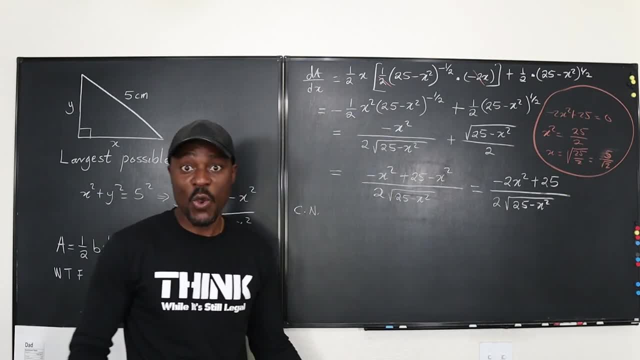 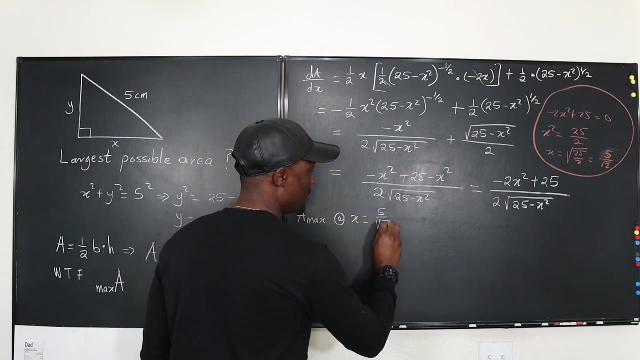 because now I know x equals 5 over the square root of 2, which is the only possible answer that I can say that a is maximum at x equals 5 over square root of 2.. So that's it. That's all you need. 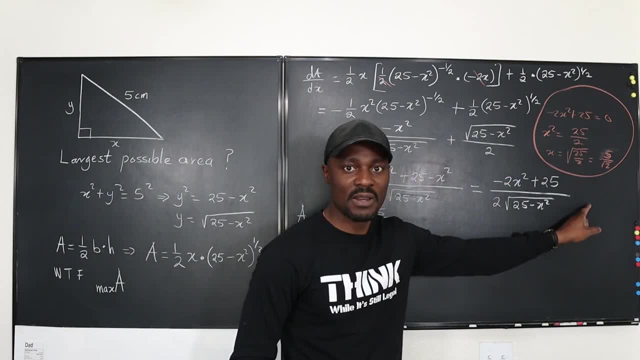 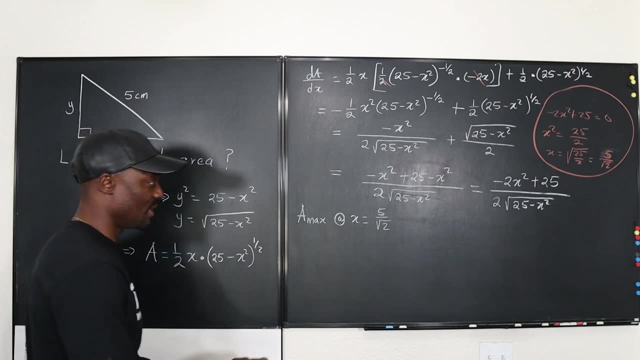 just because you were able to find the solution here. So now let's see what the maximum area. So don't stop. The maximum area is what we're looking for, the largest possible area. So what's the formula for area? again, We said the area is going to be half base times. 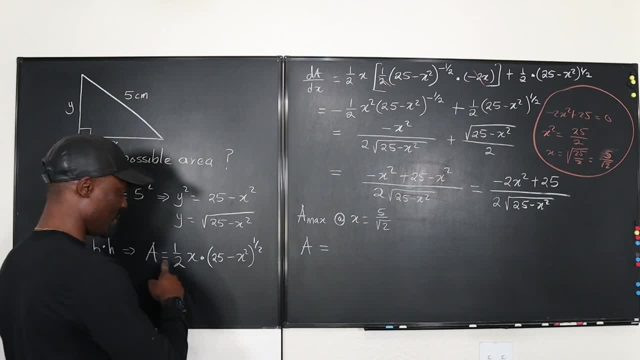 height, which you can do this, but I don't want to do this. This looks too complicated, So I'm going to say what is y? So at x equals 5, which implies y will be what. What will y be? 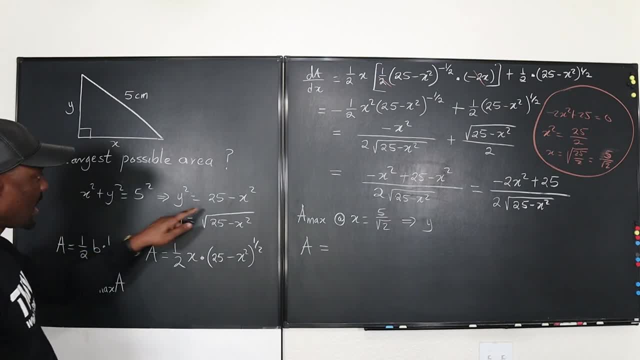 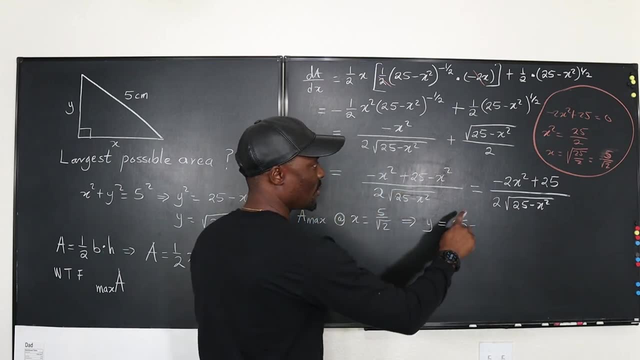 when x equals this, We said: y is 25 minus x squared equals 25 minus x squared. Oh, we already found x squared somewhere here: 25 over 2.. So I'm going to go back and rewrite, I'm just going. 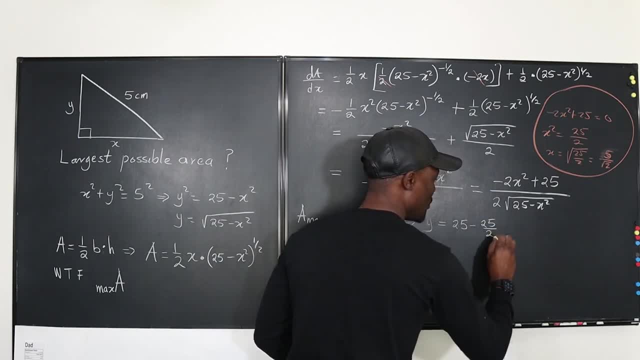 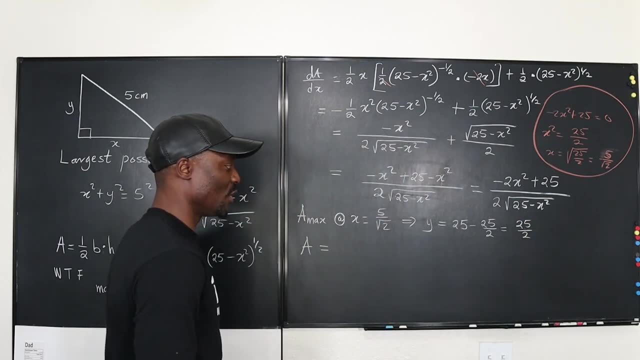 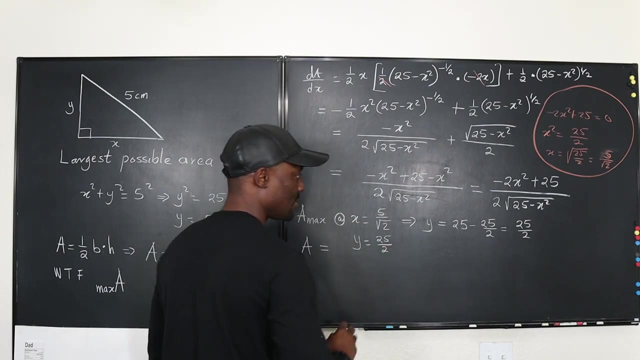 to use this: 25 over 2.. 25 over 2.. So what is 25 minus half of 25?? Well, it's going to be 25 over 2. also Simple reasoning. So now I have x to be this and I have y to be 25 over 2.. No, no, no something.